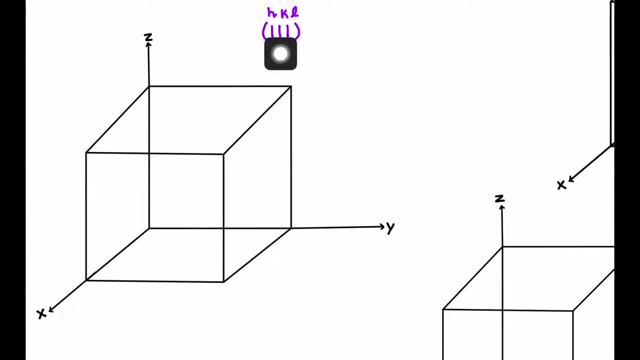 So first we have to find the point of intersection of this plane on X, Y and Z axis, And the point of intersection will be just reciprocal of the Miller indices, So it will be 1 upon 1, 1 upon 1 and 1 upon 1, that is. 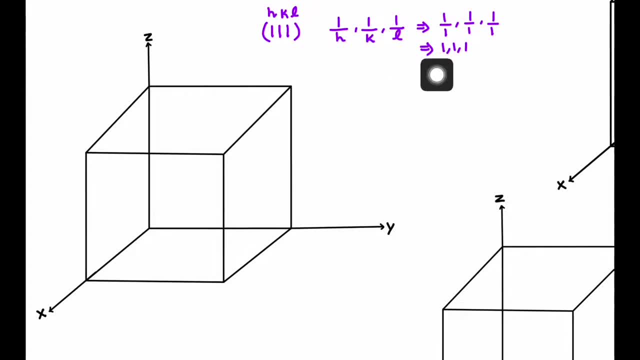 1, 1, 1.. So at X axis this plane will intersect at 1, Y also 1 and Z also 1.. So if I just represent the point of intersection along X axis, this will be the point of intersection: one unit On Y axis it will be intersecting at this point. 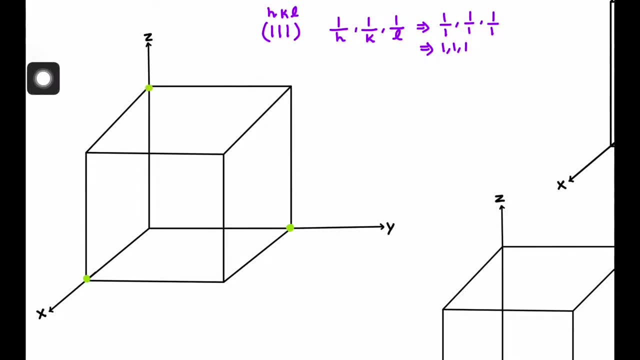 that is, 1, 1 and Z axis along Z axis. this will be the point of intersection. So now we have to simply draw the plane. So we'll simply join these points. Okay, So we will be joining this point and we'll be getting the plane. 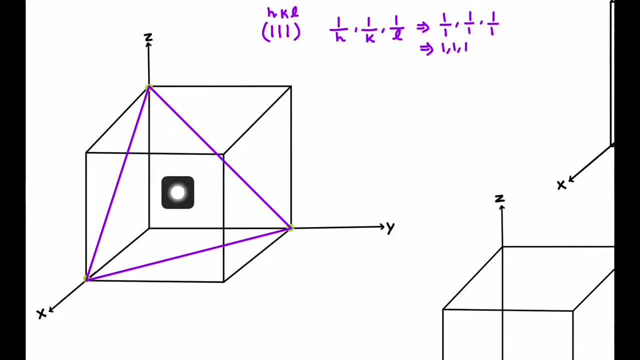 It. So that is the required plane. Let me set it for clear representation. This triangular plane basically is 1, 1, 1 plane. Okay, So this is basically 1, 1, 1 plane, Okay. 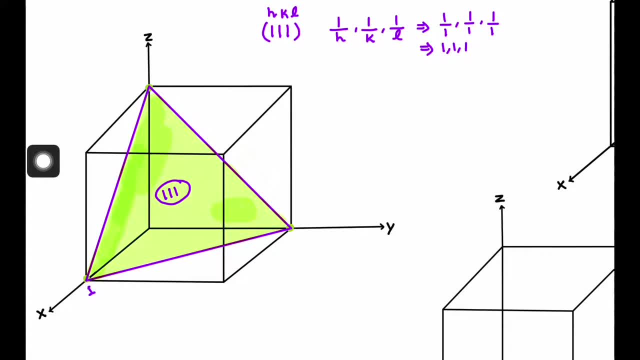 So this 1, 1, 1 plane is intersecting X axis at 1, Y axis at 1 and Z axis at 1.. And the point of intersection is simply determined by taking the reciprocal of this Miller analysis. Okay, 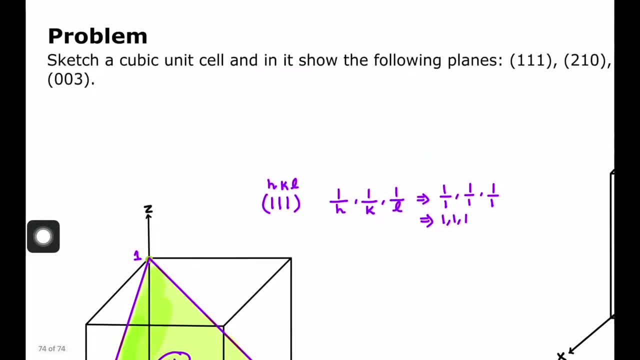 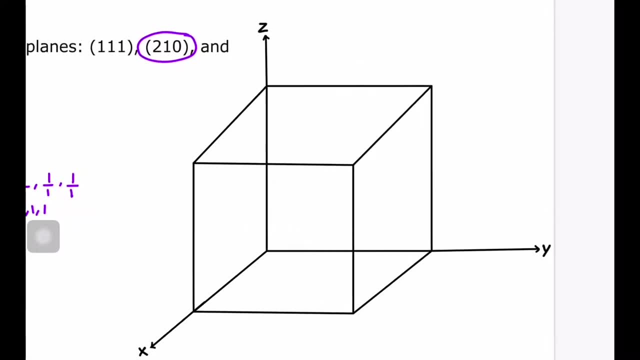 Now let's see: the next plane that we have is 2, 1, 0 plane. that is 2, 1, 0 plane, So let's draw here. The plane is 2, 1, 0.. 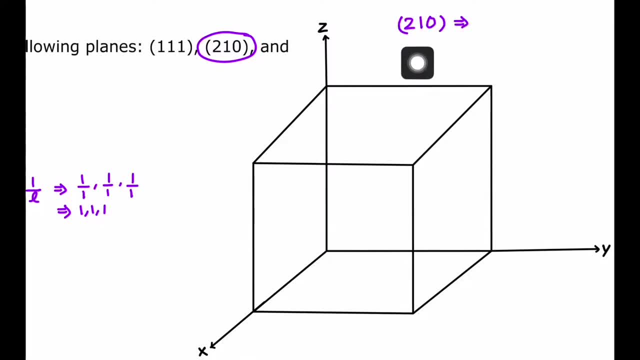 So Miller indices are 2, 1, 0. So we'll just reciprocal. We'll take the reciprocal of this to get the point of intersection at X, Y and Z axis. So it will be 1 by 2, 1 by 1.. 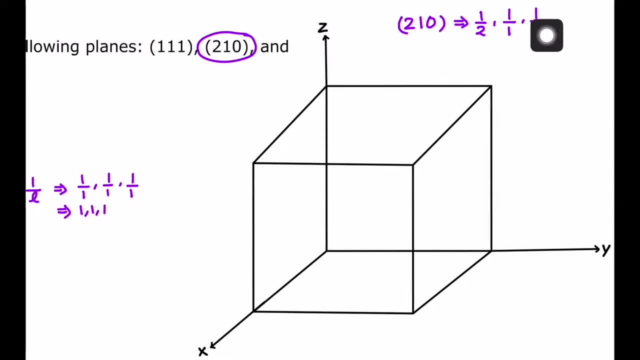 And 1 by 0, that is infinity. It means this plane will not be intersecting the Z axis. Okay, It will not intersect the Z axis. Okay, So now, along X axis, it will be intersecting at 1 by 2.. 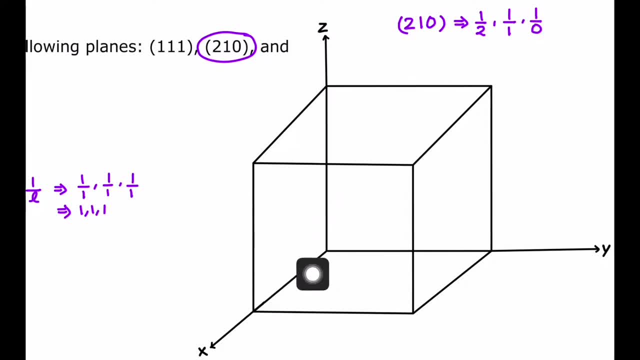 Okay, So from center to this it is a distance 1.. So 1 by 2 is just half of that. So I will make the point here. This is half of this distance edge length Now. so this is the point of intersection at X axis. 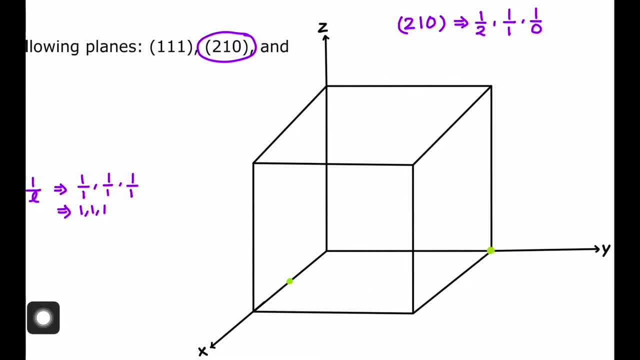 On Y axis, it is at 1.. So this will be the point of intersection. This is your origin: 0,, 0,, 0.. And Z axis it is infinity. So it is not intersecting. Okay, Okay. 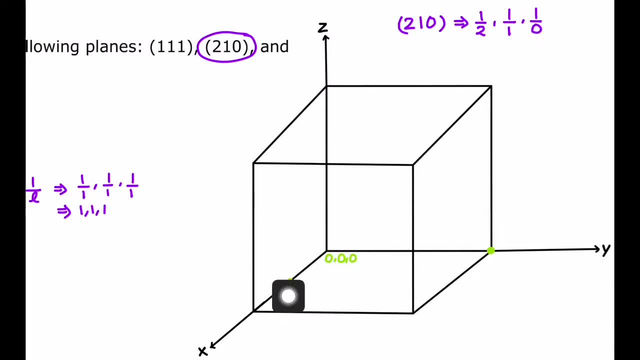 Now. so to make a plane in that, basically we have only 2 lines here. Okay, Sorry, 2 points here that will be joining, So let me. Let me join these 2 points here. Yes, But it is not a plane. 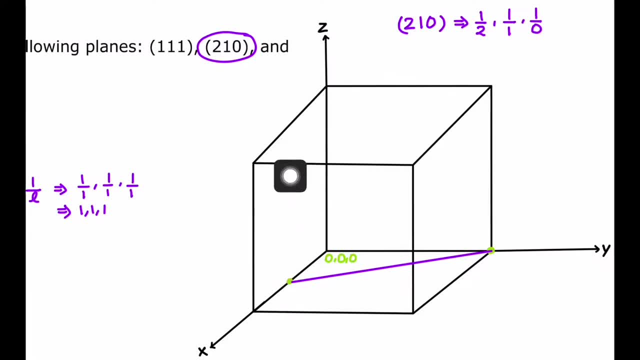 For making plane. we have to, just, you know, extend to this point here, This point, The parallel, you know sides here also, And parallel to this is that one, this point here, Now we will be joining all these points. 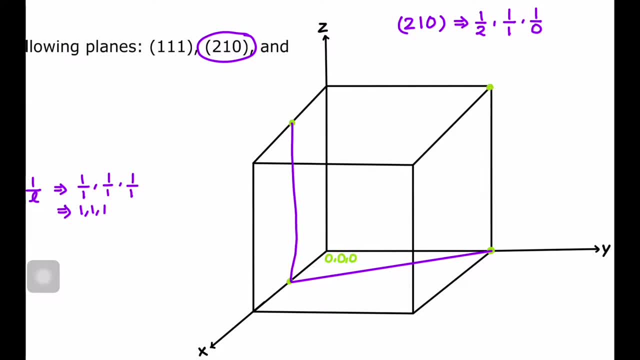 Then we will create a plane. So we are joining Now C. Now, this plane that we are getting is parallel to Z axis. It means it is not intersecting the Z axis. Okay, Because it is intersecting the Z axis at infinity here. 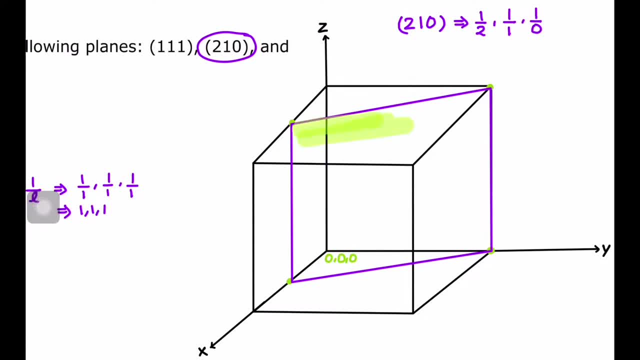 So let me set it to just get a clear view. Yeah, So this is the plane which is 2, 1, 0 plane, The shaded region. Okay, Now let's see the third plane, That is 0, 0, 3.. 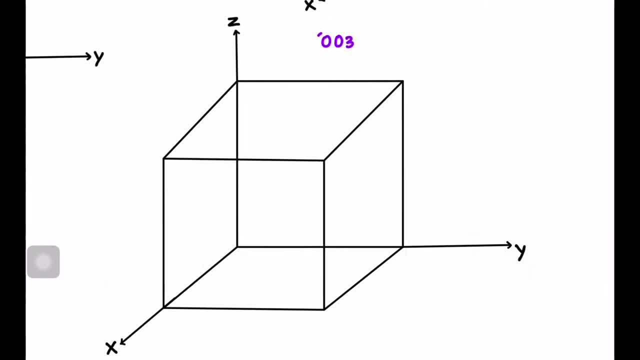 Okay, So it is 0, 0,, 3.. So the point of intersection at X axis will be 1 by 0, Y 1 by 0, and Z 1 by 3.. So it will not be intersecting at X and Y axis. 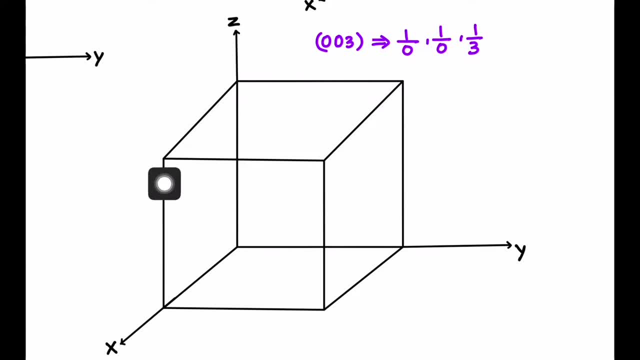 It will be only intersecting at Z axis at a distance 1 by 3.. So this corner to this center is 1.. So we will take 1 by third, So somehow here. Okay, So this is 1 by 3..